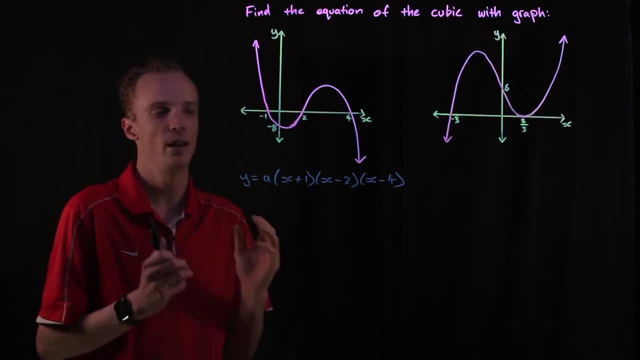 So to define this exact cubic, we need to substitute another point In another point other than the x intercepts that we've used so far. Now the point that we've been given is the y-intercept. So what that is saying here is: when x is equal to zero. 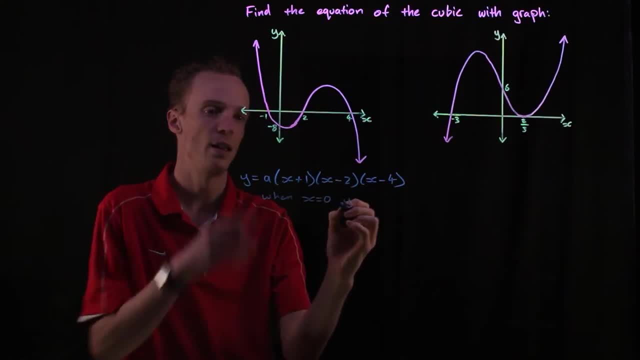 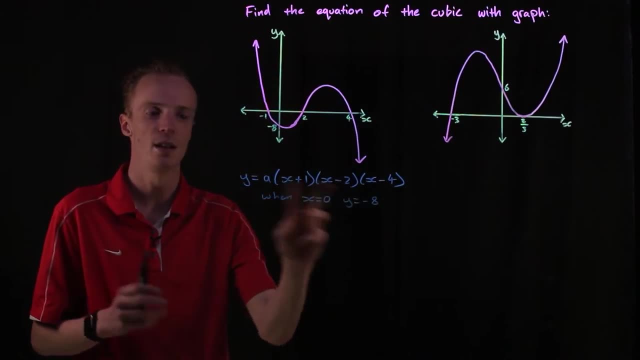 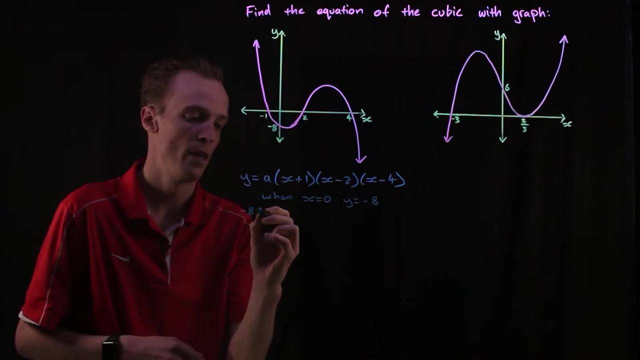 our y here is going to be equal to negative eight. So what we do essentially is we substitute these values in here and we solve for what this a value would actually be. So when y is equal to negative eight, our x is going to be equal to zero. So this will be one overall zero. take two is negative two. 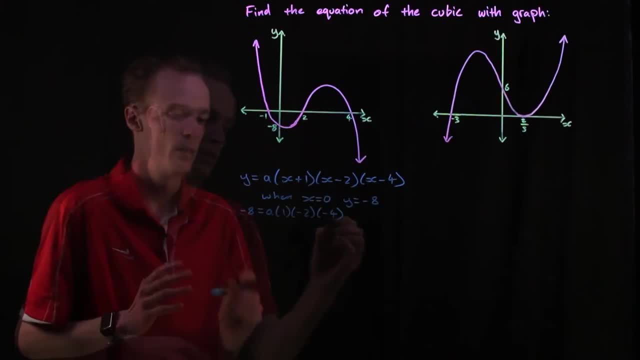 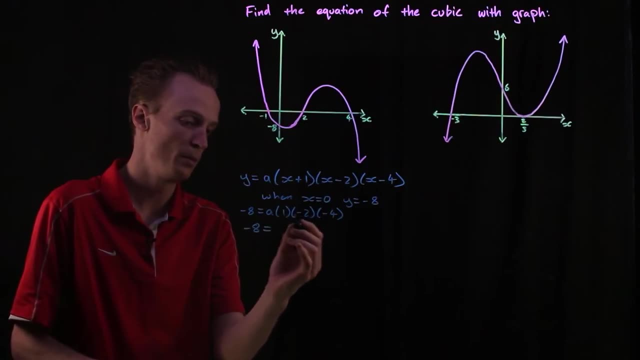 zero. take four is negative four. So from here I want to just multiply this part here out. So this negative eight here will be equal to negative times. negative will be positive, So it'll be eight a. And now dividing both sides by our eight here, we'll find that our a value is going to be equal. 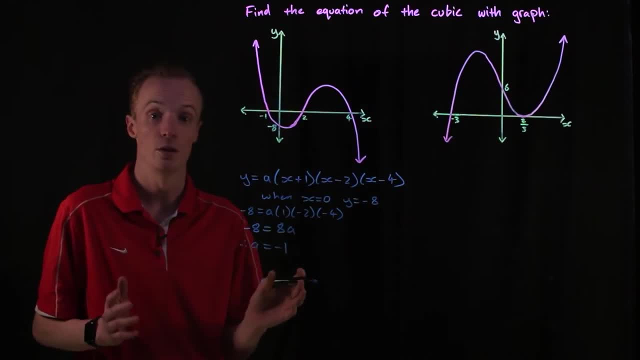 to negative one for this to be true. So what we do is we substitute this a value back into here, and we've found the equation for the cubic polynomial that's graphed here. So therefore our y will equal negative one, So which is just. 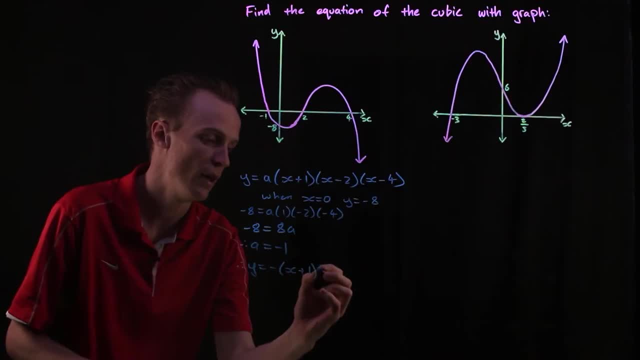 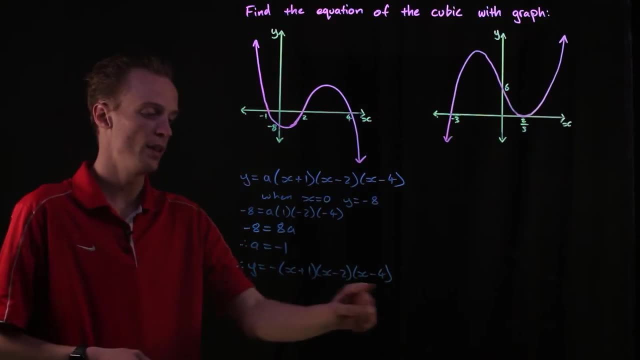 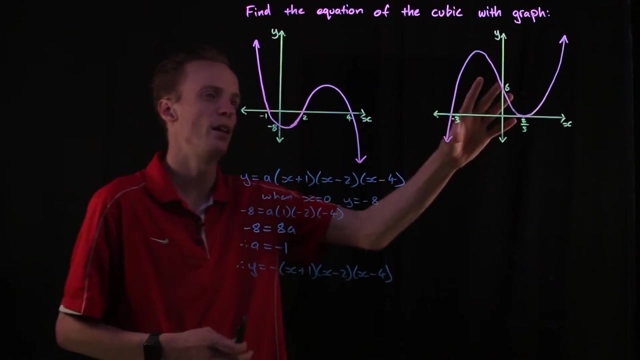 negative, our x plus one, our x take two and our x take four, So that there is the equation that represents this cubic polynomial that I've got here. So, moving on to the next point, we're going to the next one that I've got here. What's different about this one that this one here didn't have is: 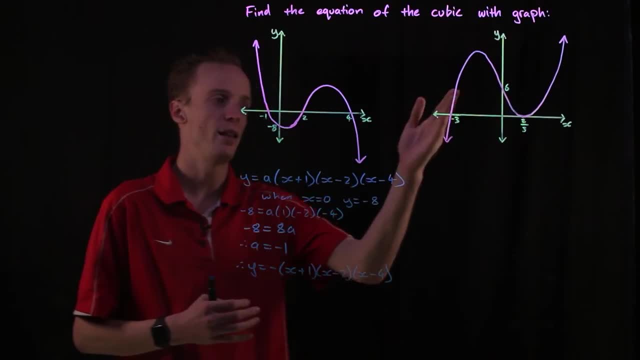 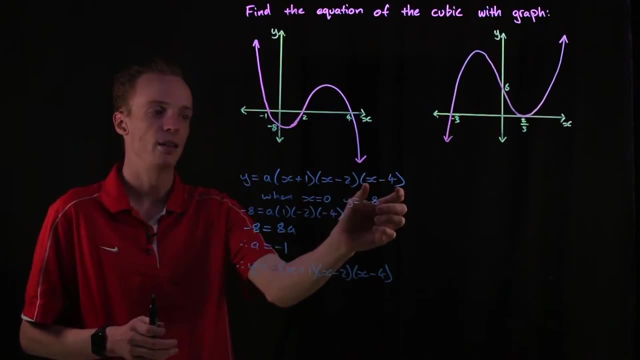 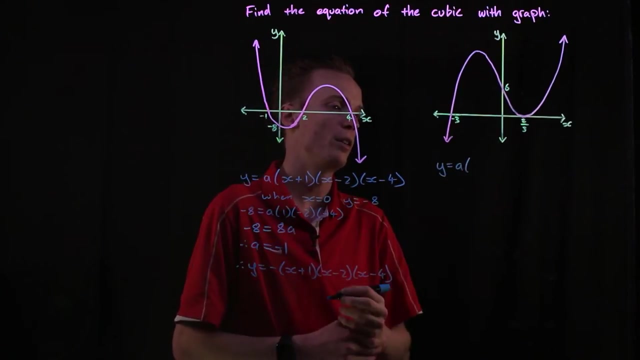 it's got a repeated root as well as a linear root. that's where it's just cutting through Now with our repeated root, we know that that's going to be that linear factor all squared. So when we're going to graph this, just generally, what we know is we've got this root here, which 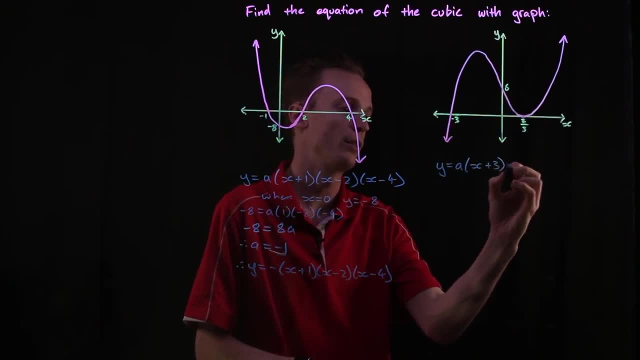 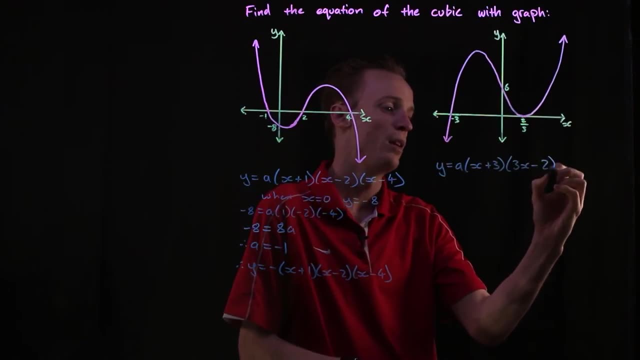 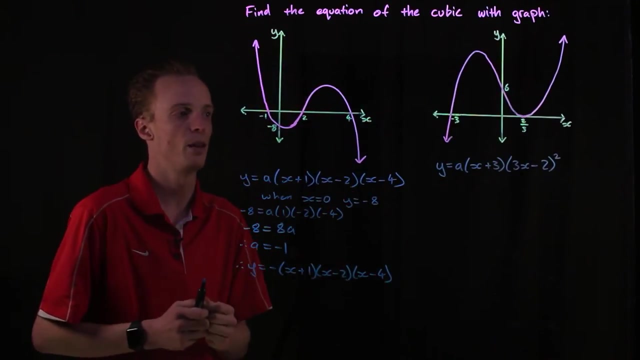 we just do what we did before, So this will be x plus three, because it just cuts through. If I just represent the linear root, so that'll be three: x take two. But because it's only touching here, we need to square this factor here And from here we follow the same sort of steps.